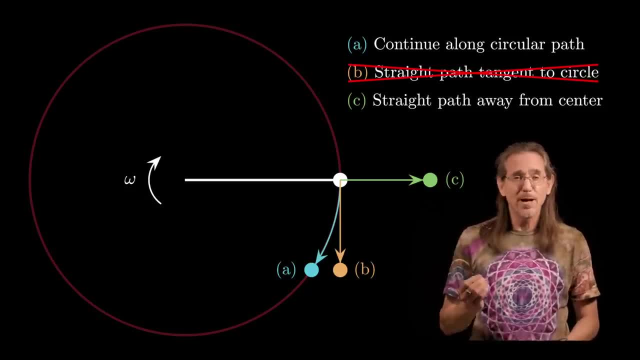 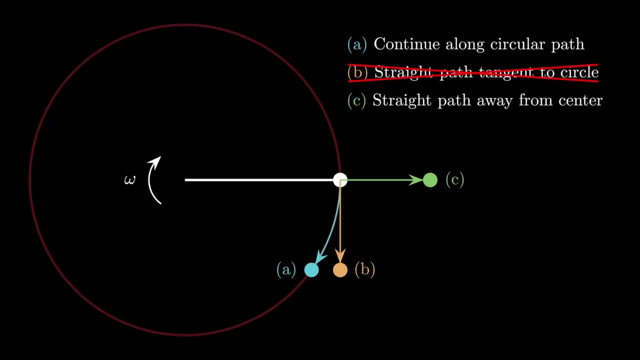 the end of this video, I'll have you convinced that another answer is indeed correct. Before discussing why answer b is incorrect, let's first take a look at answer c. Some of you might think that this answer is obviously wrong, but it's not as strange as you might think. It all depends on your perspective. 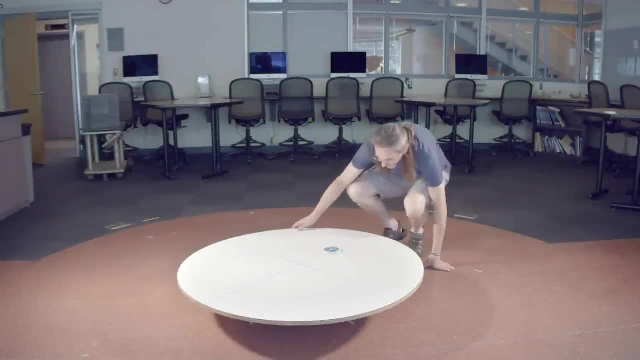 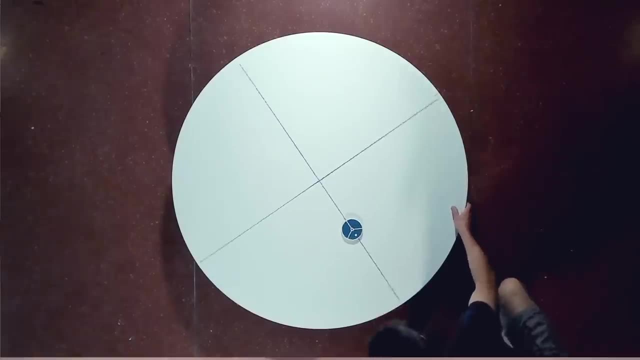 Let me explain. What you're looking at. here is a small plastic puck sitting on a platform that can rotate. Notice that as I rotate the platform, the mass moves in circular motion. This situation is similar to swinging a ball around on a string, with friction playing the role of the string. 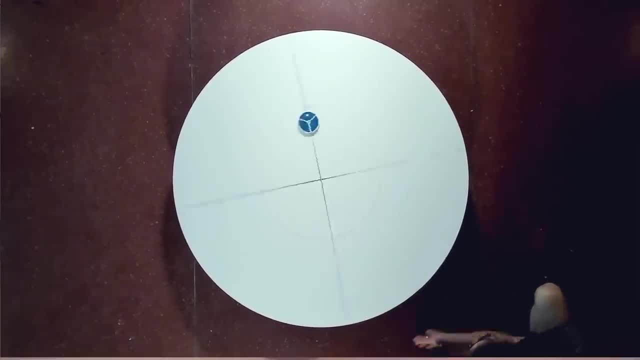 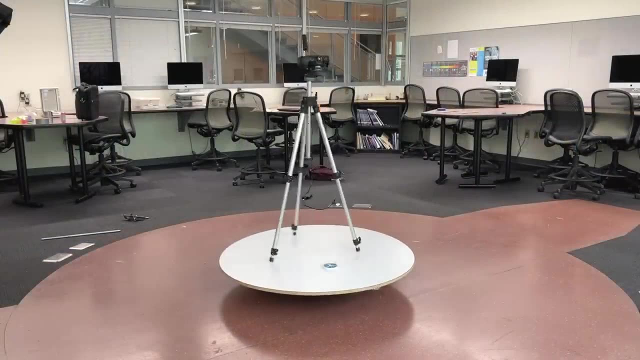 If we rotate the platform faster and faster, there comes a point when the mass begins to slide, which is similar to releasing the string. But what do we observe if we happen to be on the rotating platform Initially? the puck remains motionless. 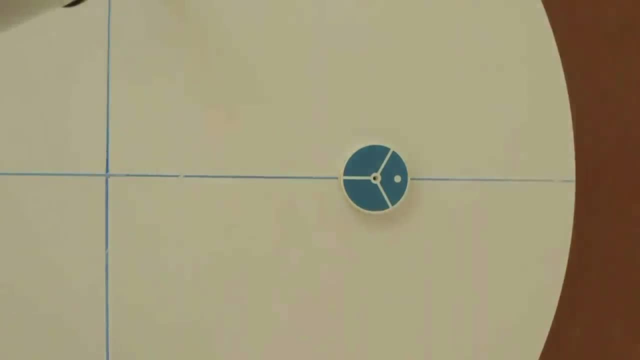 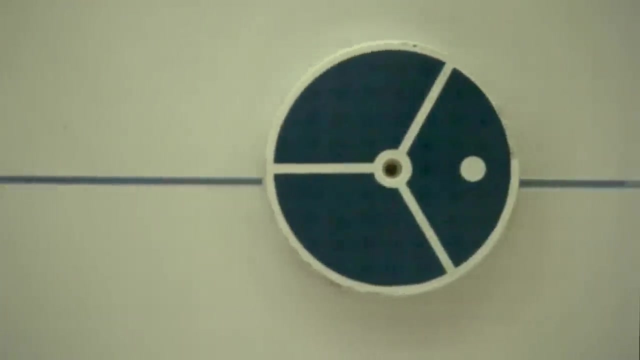 But once we reach a high enough rotational speed, we see that the puck moves away from the center of the platform and curves off to the left. Although it's a little hard to see, if you look closely it looks like the puck initially moves directly away from the center of the platform. 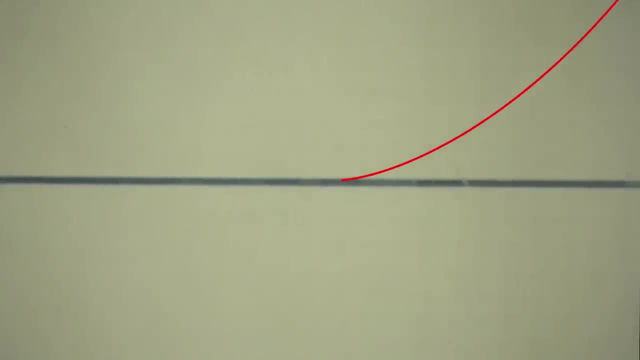 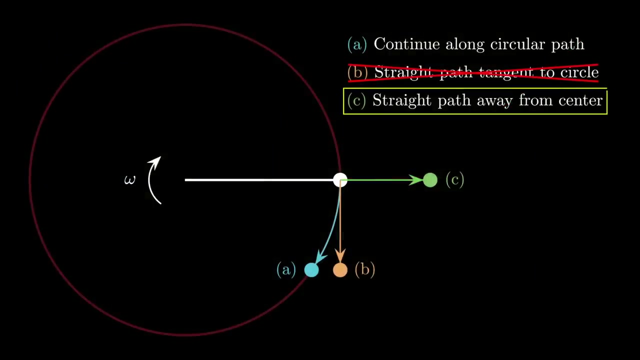 In fact, if we neglect air resistance, then one can show mathematically that this is precisely what's happening. Thus you can make a strong argument that answer c is in fact the correct answer, Assuming of course that you happen to be viewing the situation from a rotating frame. 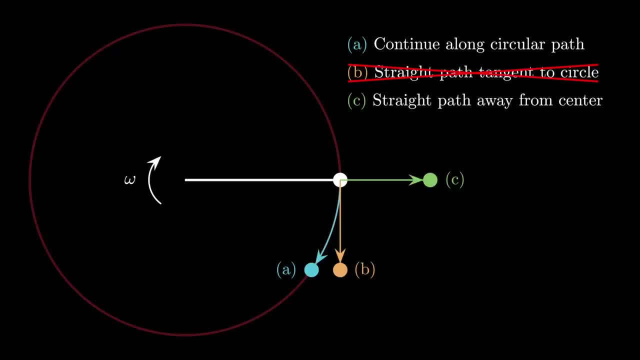 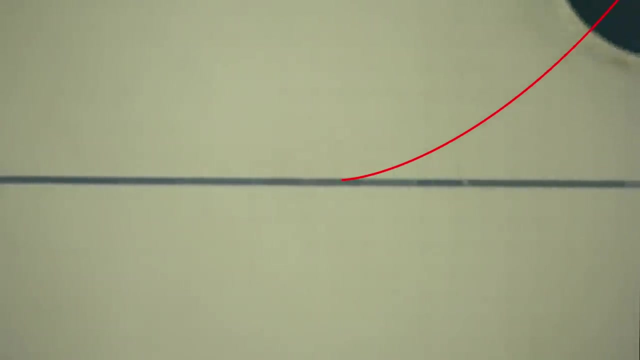 However, even in a rotating frame and neglecting air resistance, answer c turns out to be incorrect for the same reason that b is incorrect. And by now you're probably really curious why answer a turns out to be the correct answer. Before moving on, it's worth mentioning that the trajectory of the puck on a rotating platform 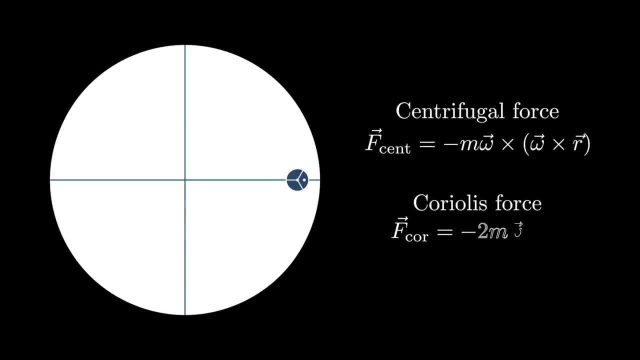 is governed by the centrifugal force and the Coriolis force, which can give rise to some very interesting motions. These forces are sometimes called fictitious forces, though this term downplays the very real effects you experience if you're in the rotating frame. 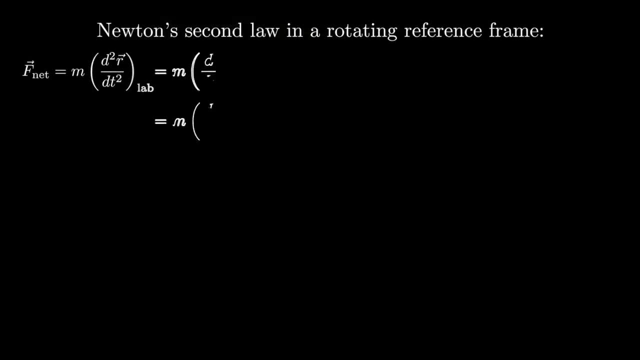 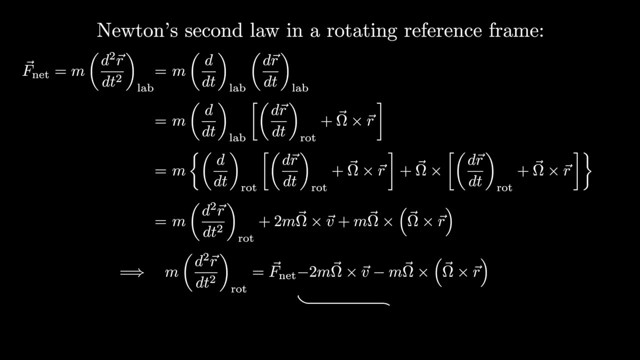 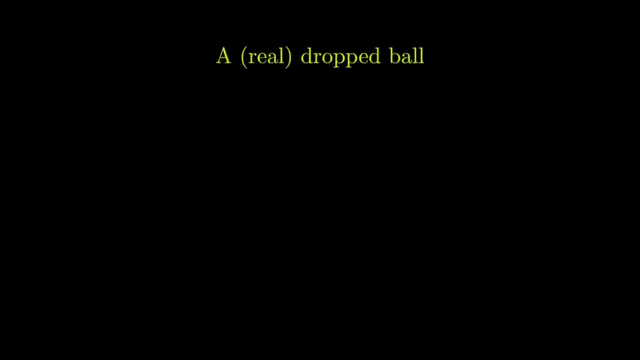 Given that we live on a rotating planet, it's actually critically important to understand how to determine the motion of an object in such a frame. The process is relatively straightforward, but the details are better left to a future video To understand why the ball continues along its curved trajectory immediately after the string is released. 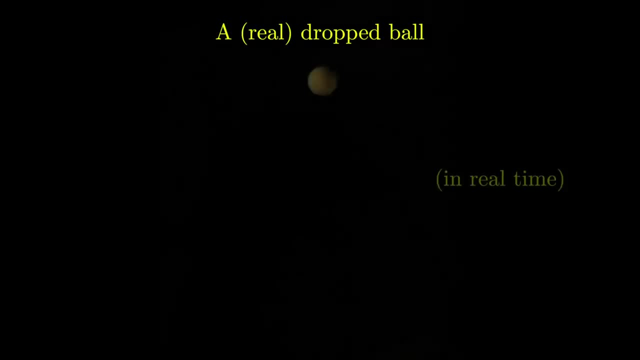 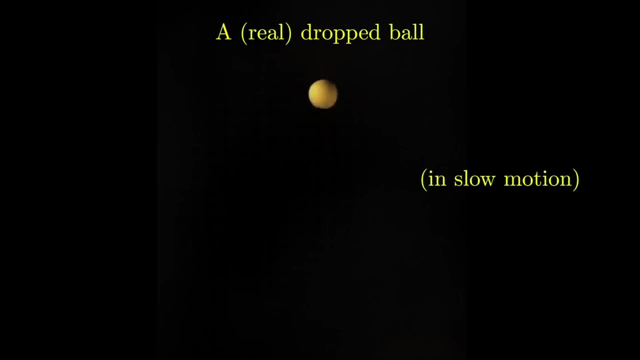 let's first think about something really simple: A dropped ball. As you would expect, there's nothing terribly interesting here. The moment the ball is released, it begins accelerating toward the ground. But things are not quite so simple if we look at a more complex object. 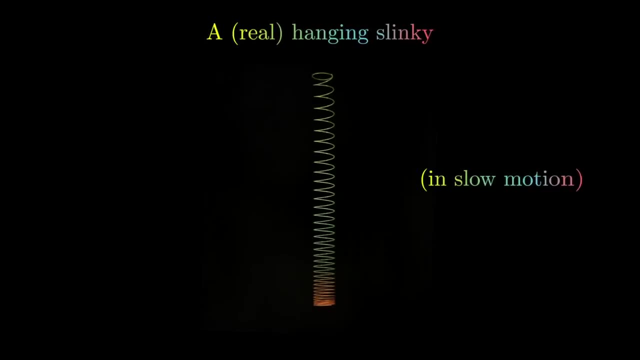 such as this slinky hanging from one end. Dropped slinkies have been very popular on YouTube, so you may already know what's going to happen, But if you've never seen it before, the phenomenon is pretty striking. Notice how the bottom of the slinky remains motionless after the top is released. 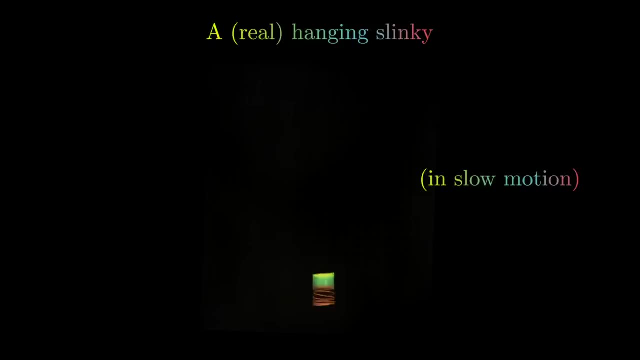 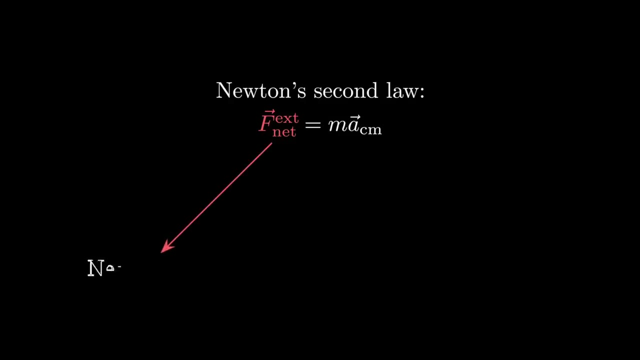 It almost appears as though the slinky somehow defies the laws of physics. It doesn't, of course. Newton's second law says that the net external force on the system is equal to the mass of the system times the acceleration of the system's center of mass. 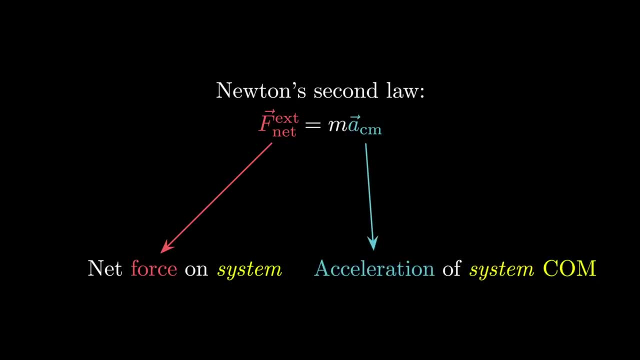 Thus, the slinky's center of mass will behave exactly like the dropped ball. To verify this is the case shown here is a slinky and a ball dropped at the location of the slinky's initial center of mass, accompanied by a simulation of a dropped. 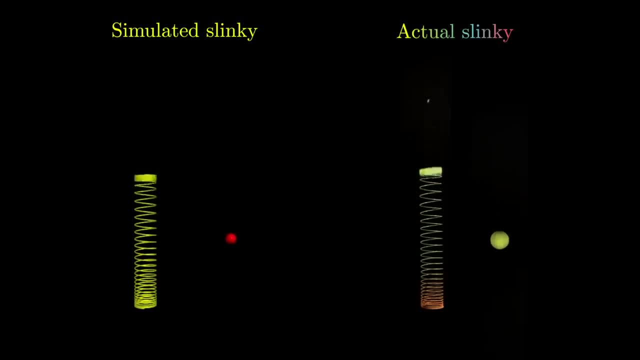 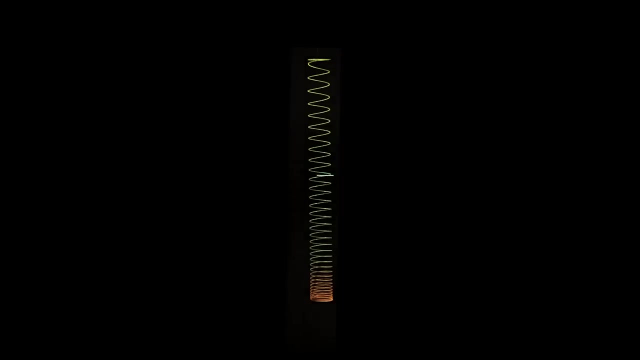 slinky, along with its calculated center of mass. As you can see, the slinky's center of mass behaves exactly as predicted by Newton's second law. What's going on here? What's causing the interesting behavior here, is the fact that there are internal forces at play. 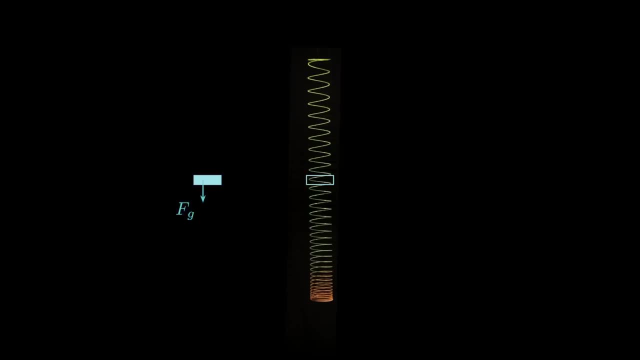 In addition to gravity acting on each coil in the slinky, there's also a tension force from the slinky itself, and the strength of this tension force is larger when the coils are more spread out. The coil spacing is thus a visual display of the tension in the slinky. 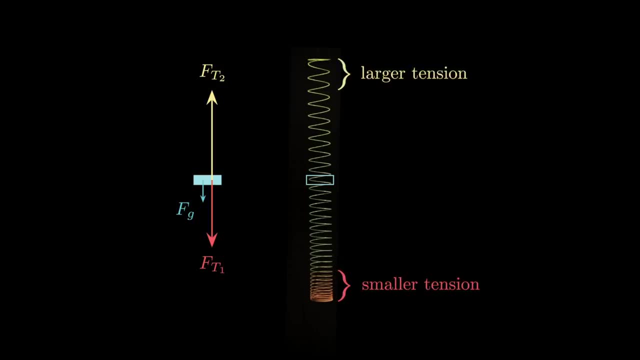 For a hanging slinky, we can see that the tension is larger near the top, which makes sense when you consider that a larger tension is needed to support a larger fraction of the slinky's total weight. Now, before the slinky is released, the forces are balanced and each point of the slinky is in. 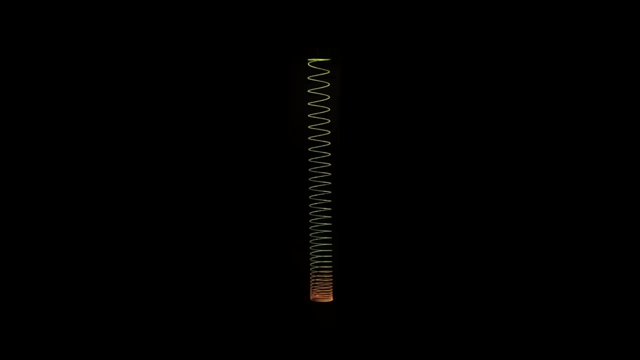 equilibrium, But once released the forces at the top become unbalanced. so the top of the slinky begins to accelerate. This acceleration leads to a change in tension that then propagates through the slinky as a longitudinal wave. Each point on the slinky remains in equilibrium until the tension wave arrives. 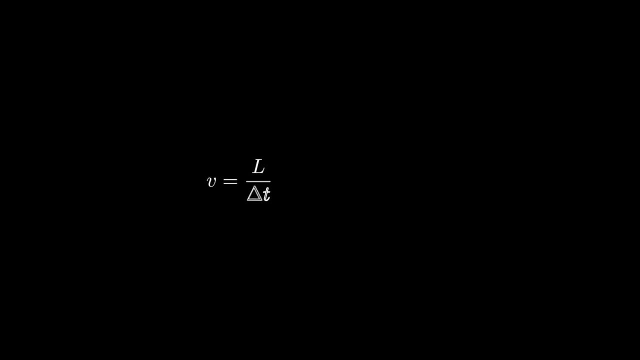 For a slinky, this wave speed appears to be roughly constant and in our particular case, we find an approximate speed of 3.3 meters per second. Interestingly for a slinky, the motion of the collapsing coils and the motion of the 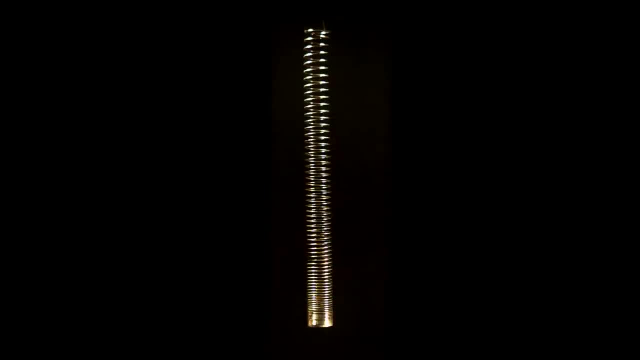 tension wave appear to coincide almost exactly. Thus the collapsing coils essentially mark the position of the tension wave. There's no reason this has to be the case. so the motion of a dropped slinky is somewhat special in this regard and may very well be one of the reasons why dropped 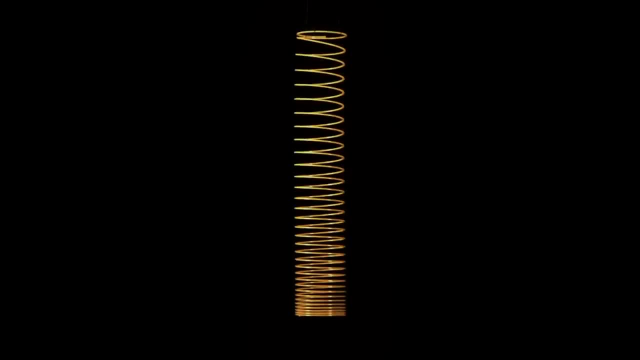 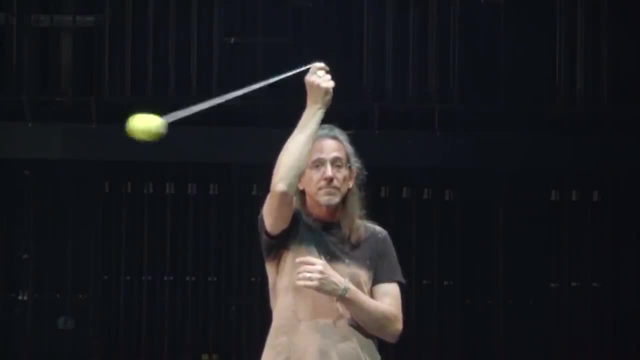 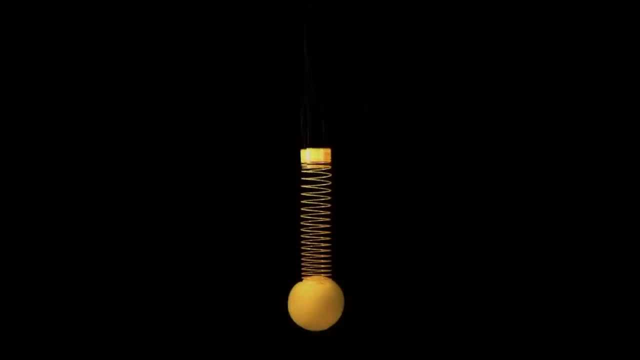 slinkys are so beautiful to watch. We'll return to this interesting point later in the video. So what does all this have to do with the question about circular motion? Well, imagine connecting a ball to the bottom of the slinky. Not surprisingly, the same phenomenon is observed. 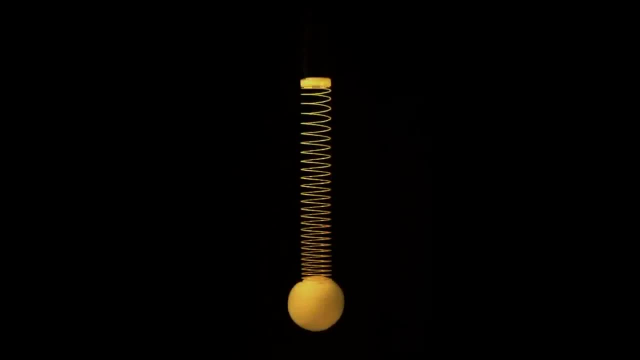 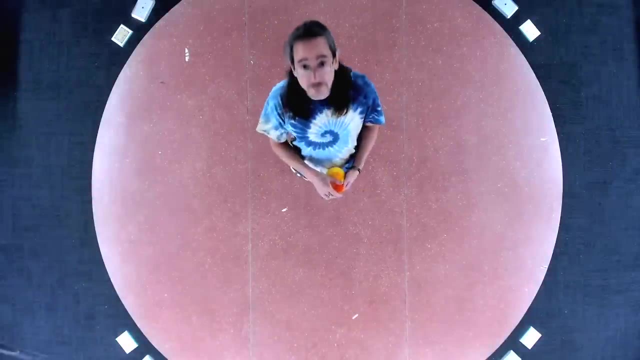 I don't know about you, but even though this behavior is expected, I still find it pretty extraordinary to see the ball levitating in the air like this. But if we now imagine the ball being swung around in circular motion on the end of the slinky 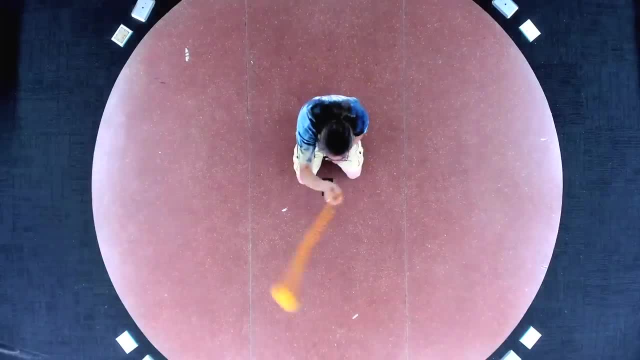 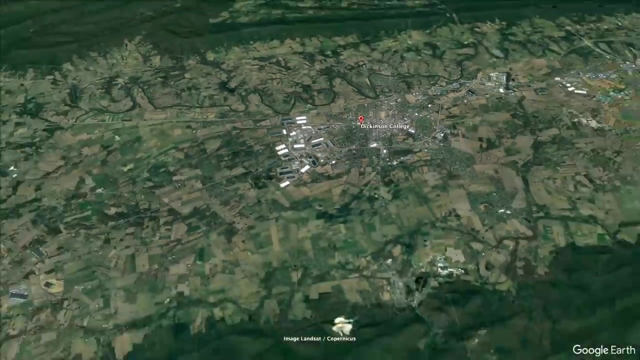 then what happens when the slinky is released? Will the ball remain moving in circular motion while the tension wave propagates through the slinky? Somehow, this just doesn't seem possible. In order to answer this question, we traveled to High Point University in North Carolina. 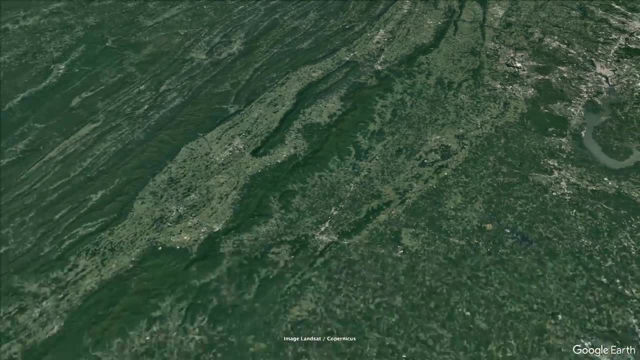 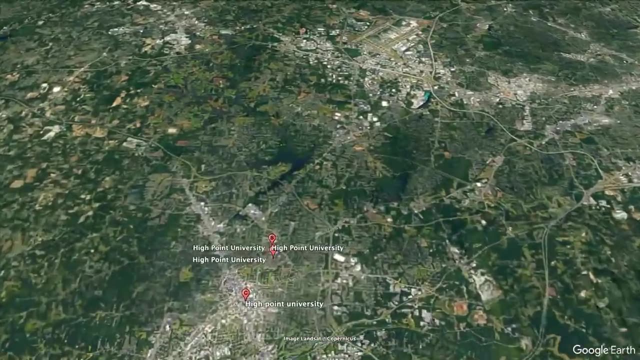 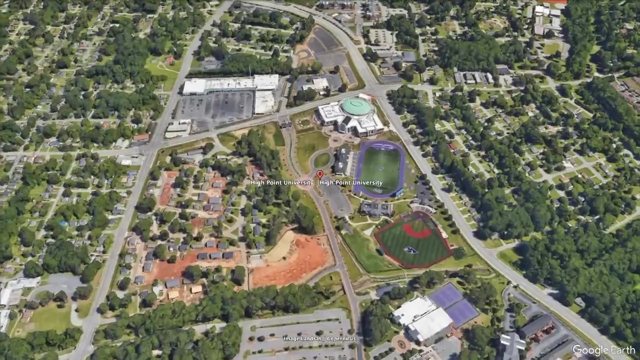 to meet up with some colleagues who had previously investigated this situation. The setup is not trivial, because you need to mount a high-speed camera well above the experiment, which then requires a lot of light. Fortunately, we were given access to the university's theater, which was an ideal. 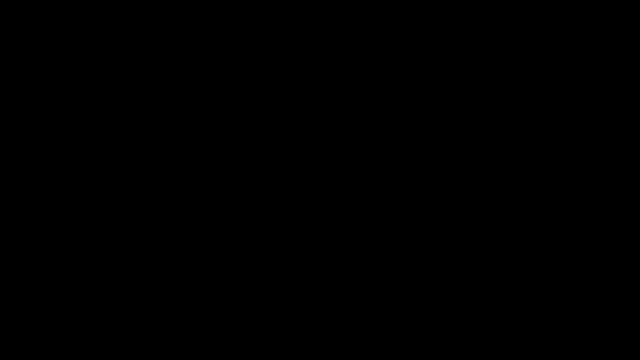 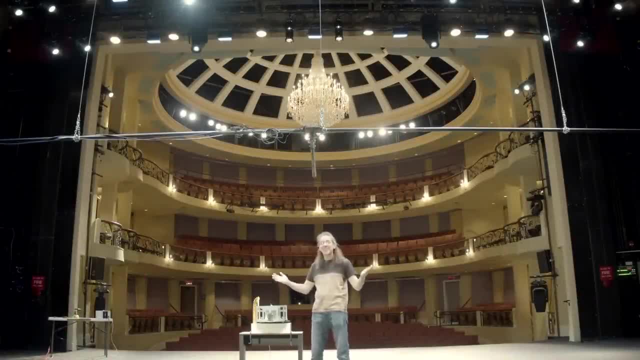 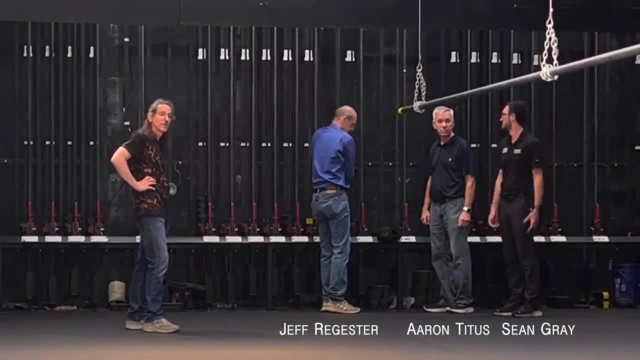 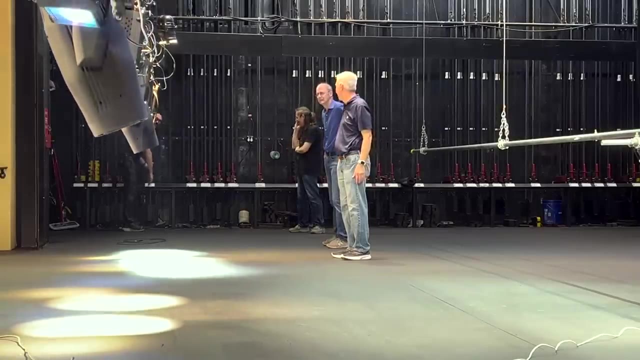 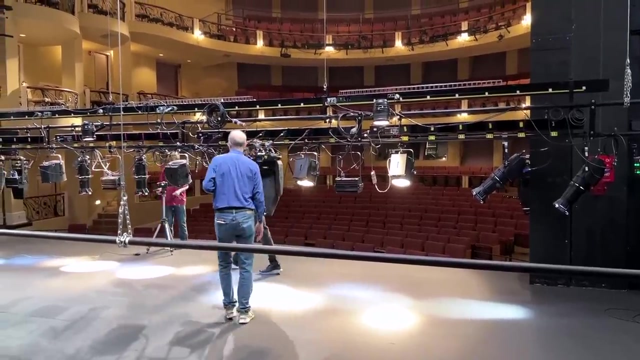 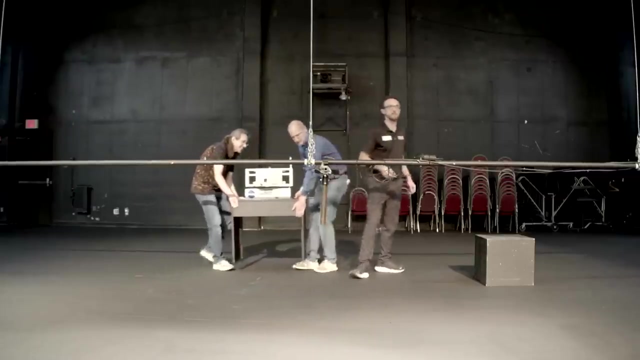 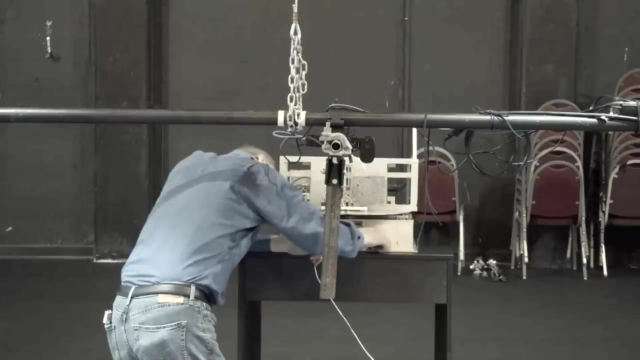 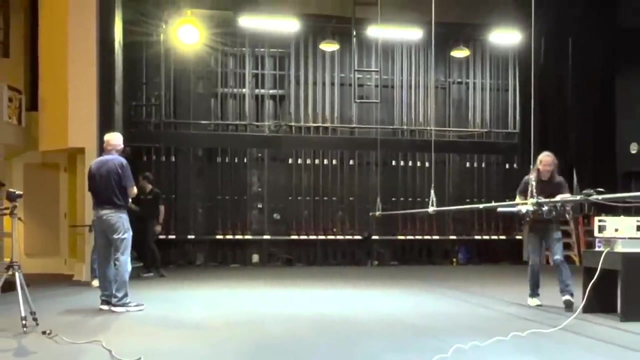 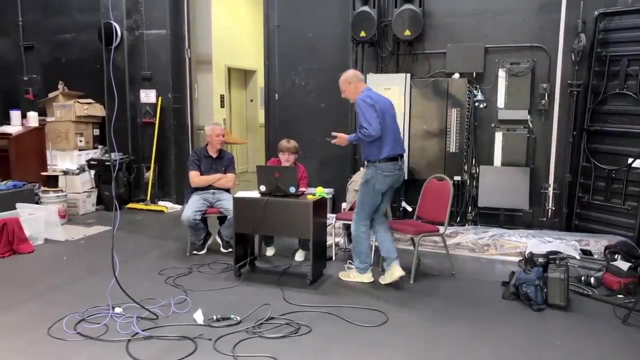 Wow, Can you believe it? This is going to be perfect. One of the reasons for traveling to High Point University is because they have a mechanical device that can be used to spin things around and release them with the press of a button. Here's Jeff Register explaining how it works. 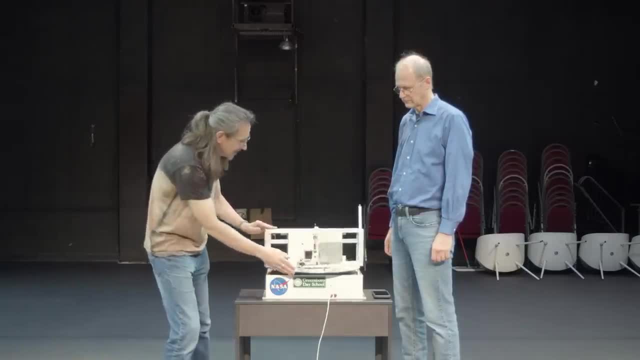 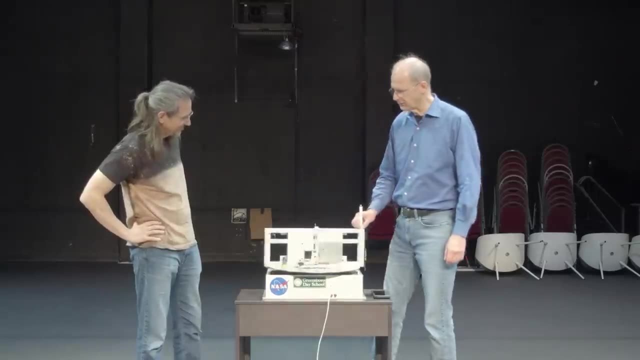 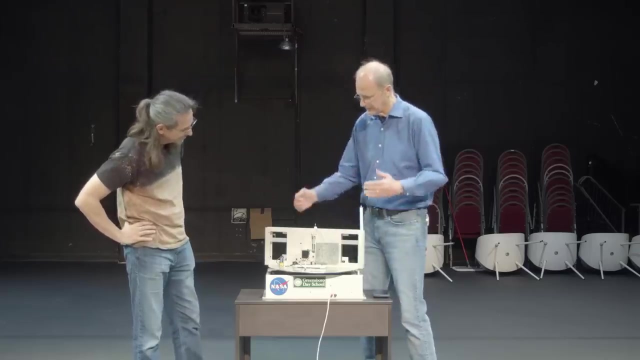 So basically the whole reason we're here is to use this really cool contraption. Can you explain how this works? Yeah, it's a turntable, So it spins around up to about four revolutions per second And under control from my phone- the electronics here- it can do various things. 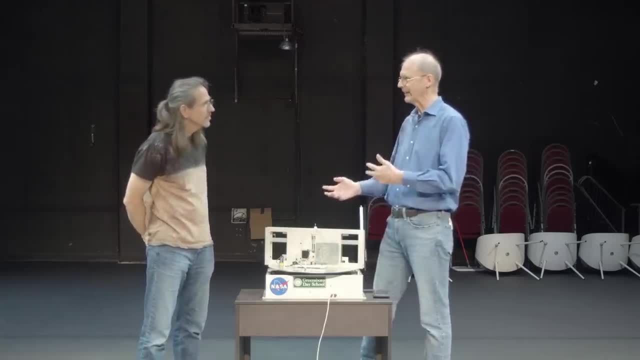 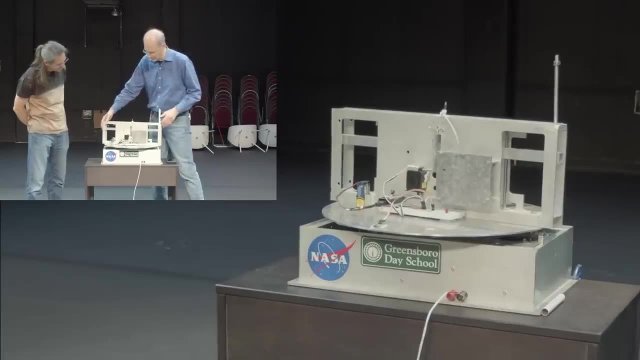 And what we're going to use it for today is to release a spring While the whole thing's spinning. we're going to release a spring, And it does that By a little servo motor. here it pulls out and releases a spring-loaded bar which drops. 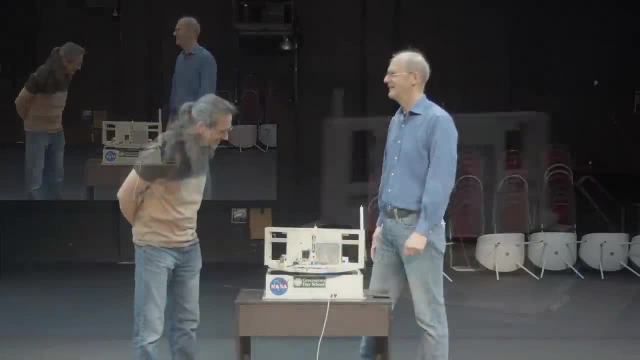 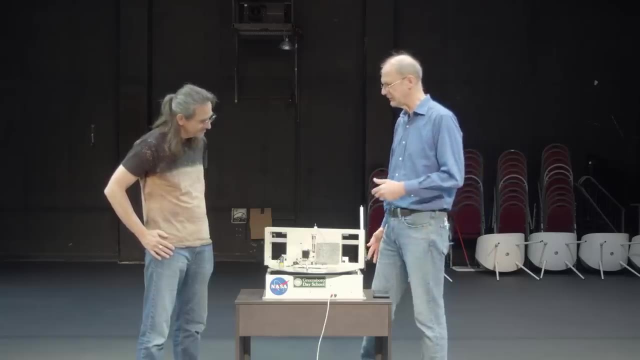 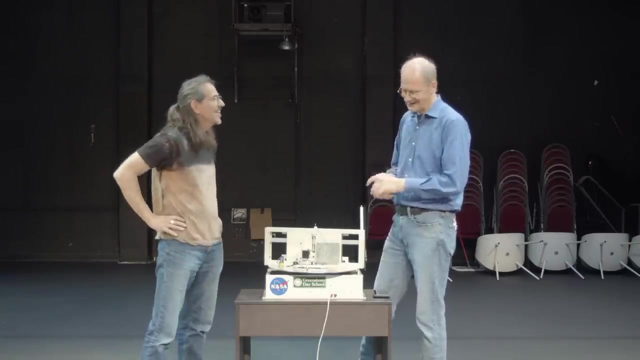 This bar will drop releasing the object. I get it And you built this from scratch. right, I did Some years ago. I built it because I put together a team. NASA had put out a call for proposals for experiments to fly on their zero-gravity aircraft. 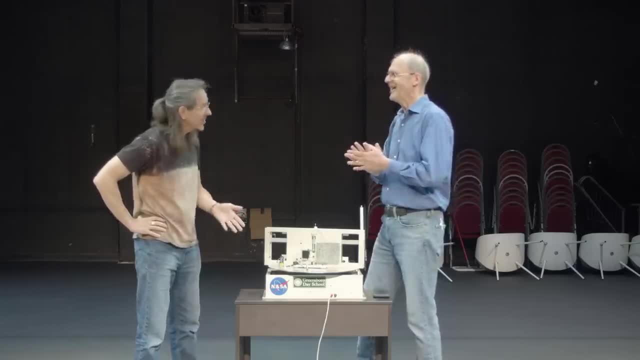 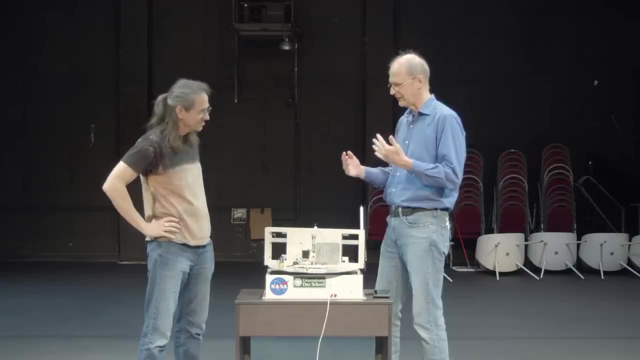 That's why the NASA sticker there. Did you actually, When I built it, NASA didn't build it. Did you actually fly on that? I did That zero-gravity airplane. this is that airplane that does the parabolas, But this got to fly and I got to fly on the zero-gravity aircraft. 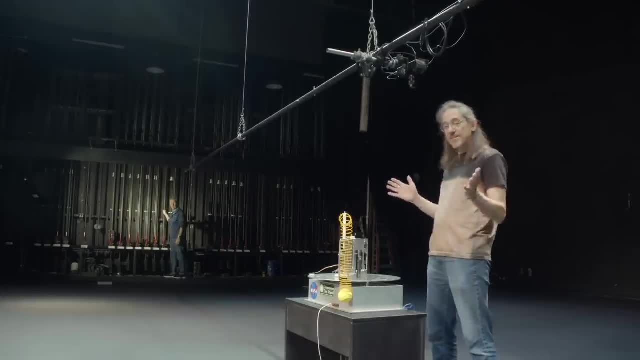 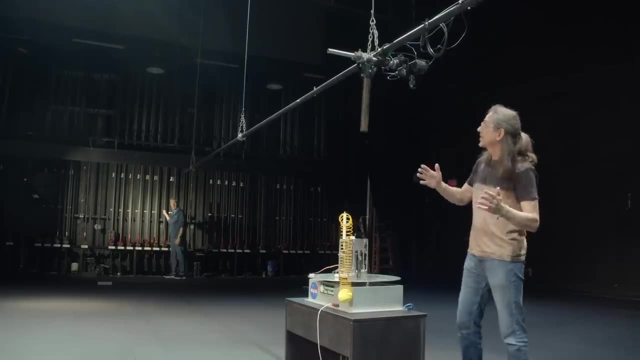 That's cool, Yeah, Okay. So I think everything's basically set up The way this is going to work. we've got the rotating table here with the slinky on board, And on this batten we've mounted a high-speed camera facing straight down to film this from. 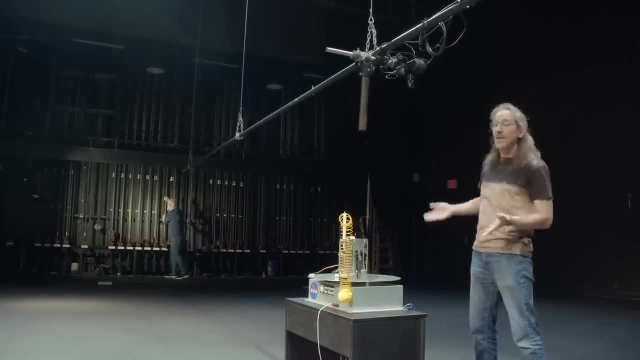 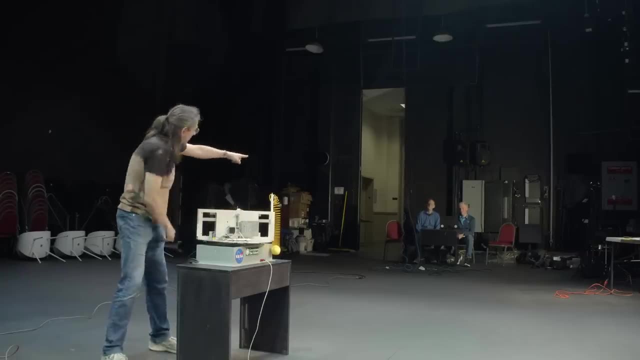 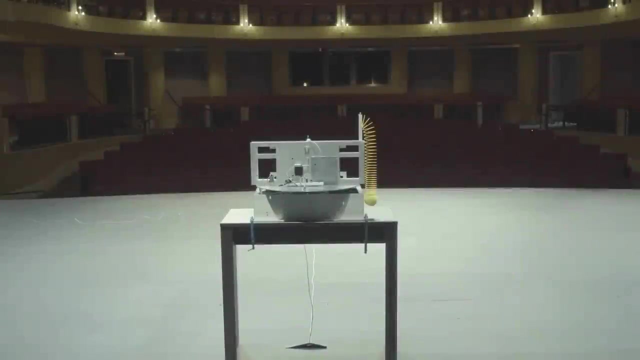 above And the batten can be moved up. It can be moved up or down as needed. Meanwhile, the camera is connected via these cables that go over to this computer workstation, allowing us to control everything remotely. Now that everything is ready to go, it's time to observe what actually happens. 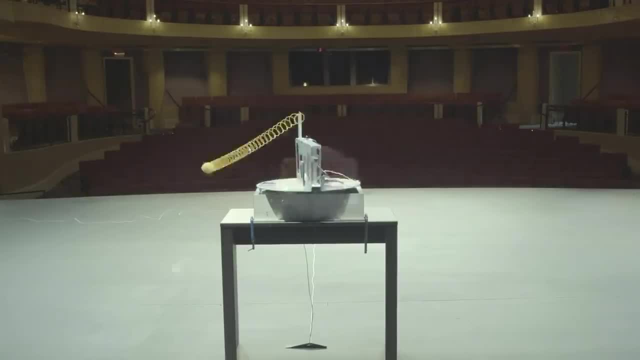 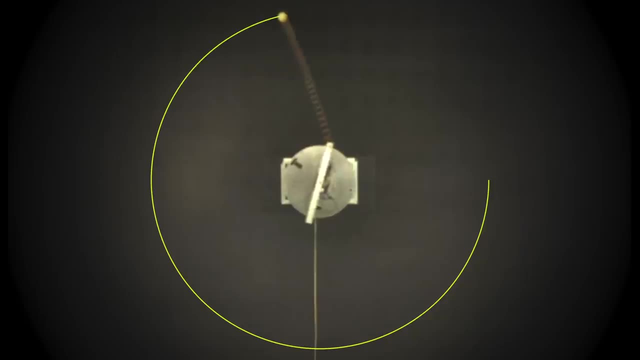 Here's a ball being swung around on the end of a slinky. Viewed from above, it's clear that the ball's trajectory is indeed a circle. It's a circle, But notice how the slinky is angled backward from where you might expect and does not point. 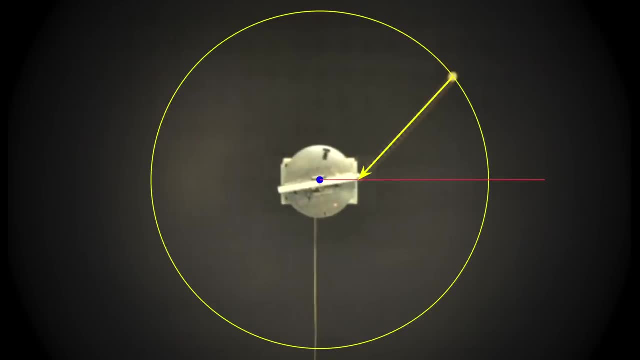 to the center of the circle. This is due to a non-negligible air drag. This drag angle results in a tension force that has both a tangential component to balance air drag and a radial component that supplies the force needed to maintain the centripetal. 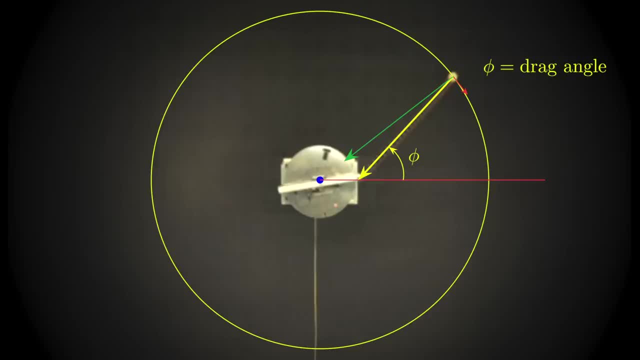 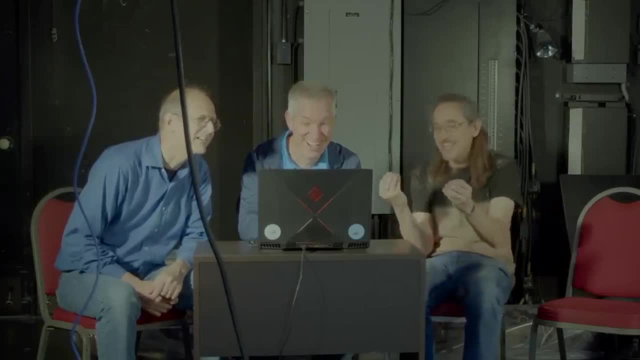 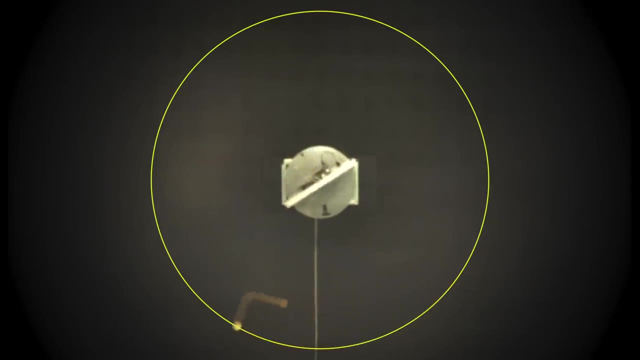 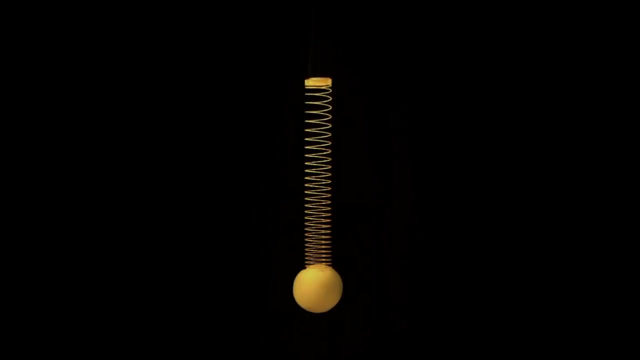 As is evident in this video, when the slinky is released, the ball continues moving in circular motion until the tension wave has traveled all the way to the end of the slinky. Although this phenomenon is essentially the same as what's happening with a dropped slinky, most people find it even more surprising to see it happen when the net force on the ball is not zero. 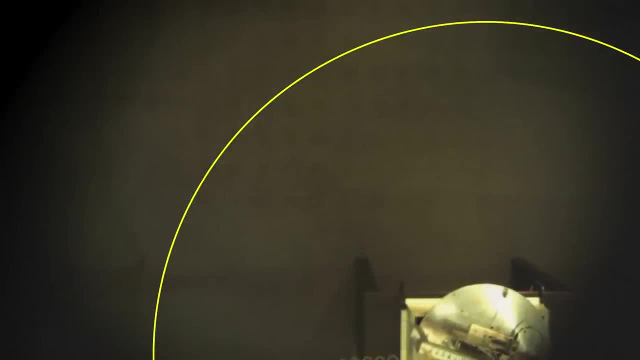 But even if you understand what's going on and fully expect the ball to continue moving in circular motion, it's still quite remarkable to actually see it play out in a real physical system. I mean, come on, You've got to admit that this is. 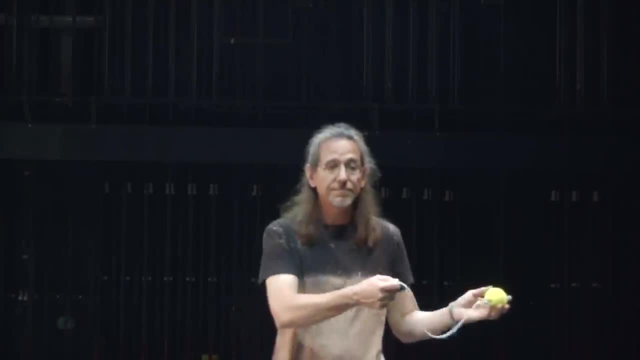 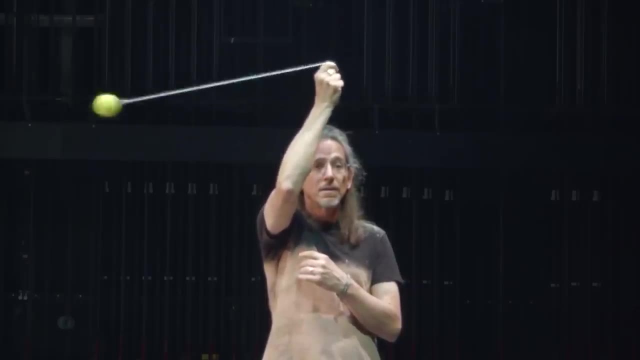 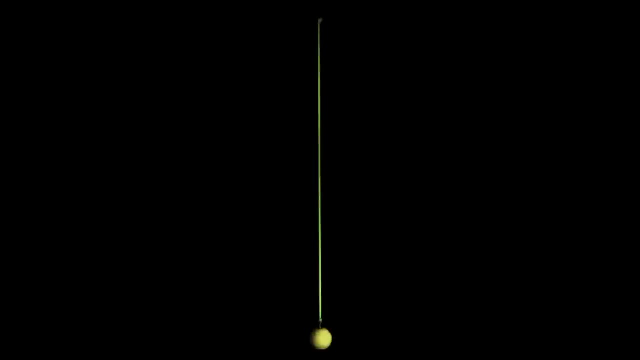 pretty amazing. Of course, the original question discusses swinging a ball around on a string, not a slinky, So let's consider something a little more string-like. Shown here is a weighted tennis ball hanging from a colorful stretchy noodle made of thermoplastic rubber, Just like the slinky. when the 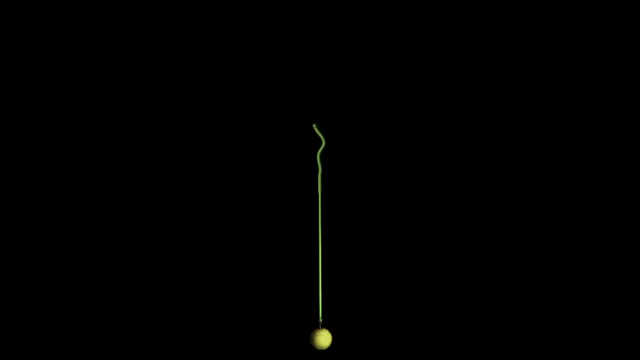 noodle is released, the ball remains motionless for a short time as the tension wave propagates to the bottom. In fact, if you watch carefully, you can see something really interesting going on. It's a bit easier to see if we orient. 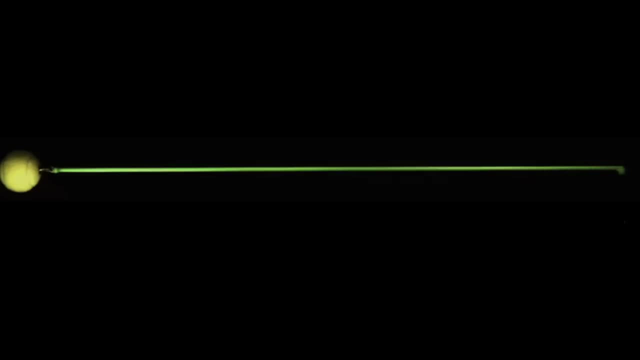 the video horizontally. Notice that when the noodle is stretched it becomes thinner, So you can actually see the tension wave propagate as a change in thickness. Interestingly, unlike the slinky, the tension wave propagates more quickly than the noodle itself, and this speed is much faster than the tension wave in the slinky And 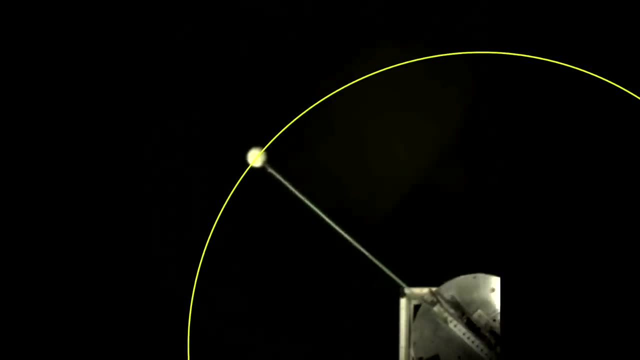 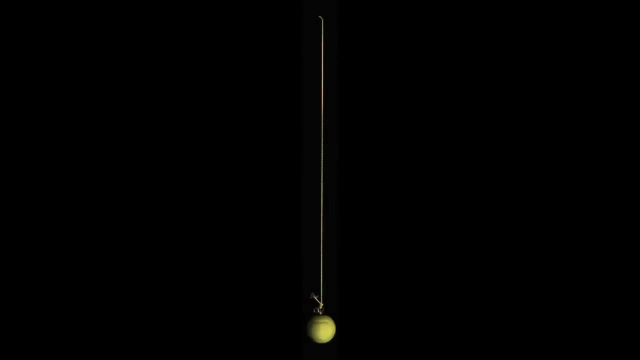 of course, if we swing the ball around in circular motion, we shouldn't be surprised to see that the ball maintains this circular motion for a short time. We can take things one step further and look at something even more string-like, such as an elastic cord. The speed of the tension wave is even faster in an 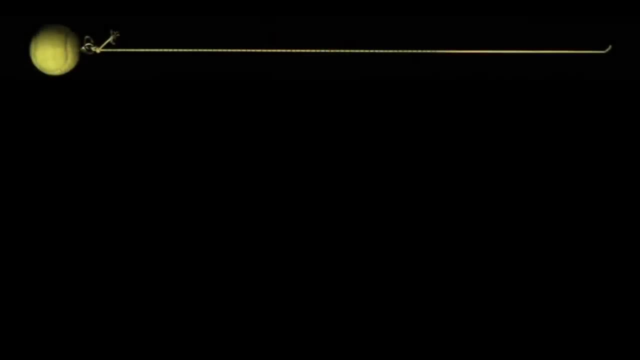 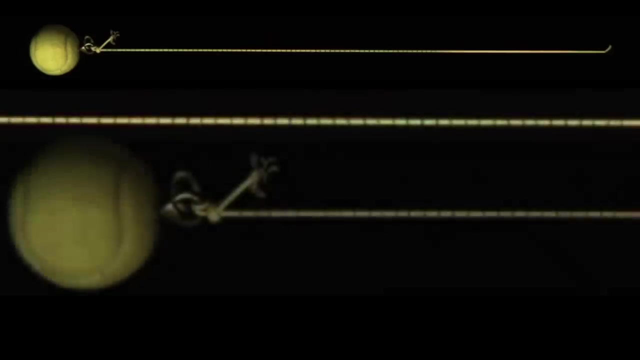 elastic cord so it's more challenging to observe. Here I've again oriented the video horizontally and I've also zoomed in to show a section of the cord that has lines drawn on it. Even still, things happen very quickly, so it's helpful to 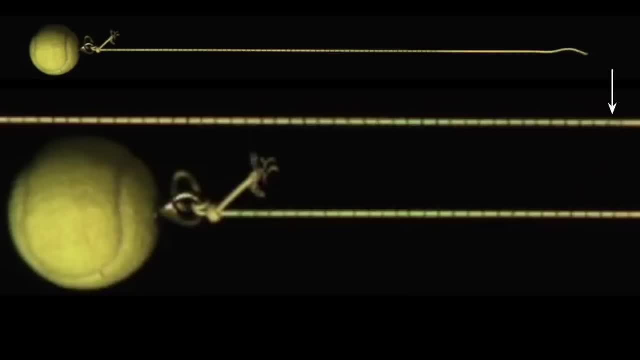 slowly step through the video to see if the tension wave is even faster. If not, you can pause the video to see exactly what's going on. If you watch carefully, you can see the lines on the elastic cord become blurry as the tension wave. 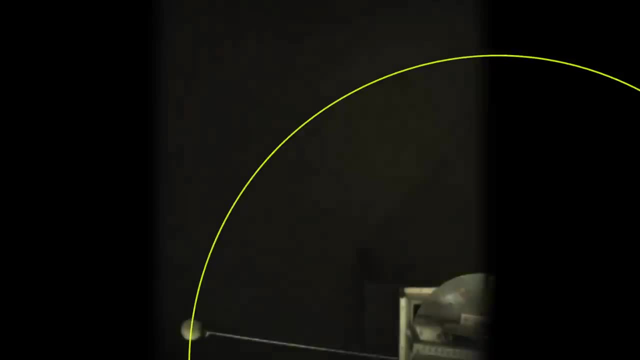 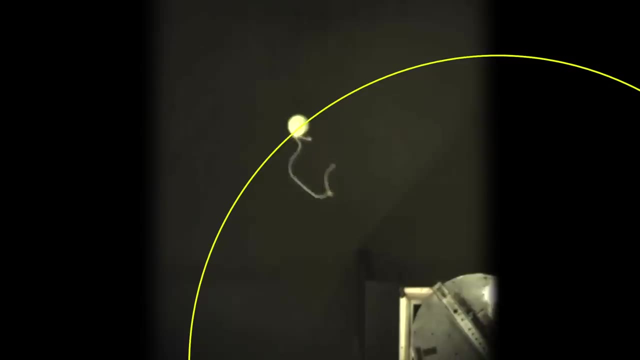 passes by And thus, just like with the slinky and the noodle, when the ball is moving in circular motion and the cord is released, the ball continues in circular motion for a brief period of time. We can do the same thing using a 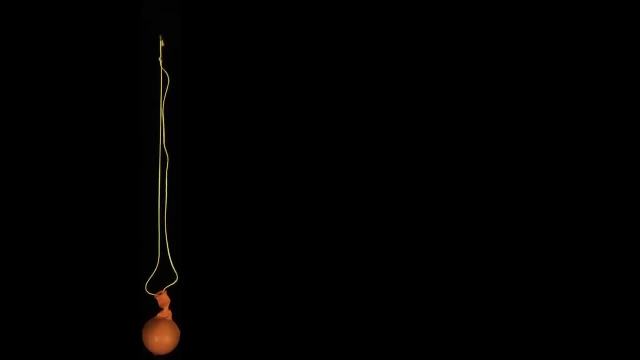 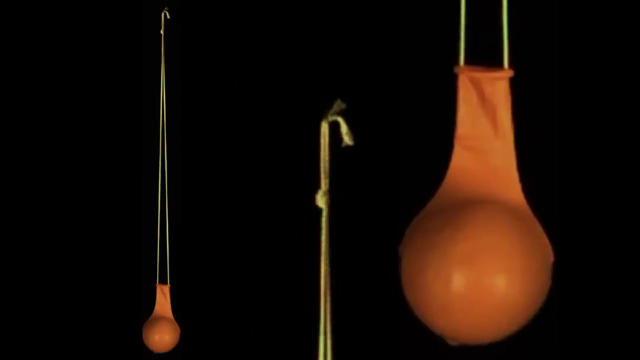 string, but the tension wave moves so fast that it's very difficult to capture. Here's a mass hanging by a string and covered by a balloon to make it easier to see. If we step through the video frame by frame, you can see there's a tiny bit of motion. 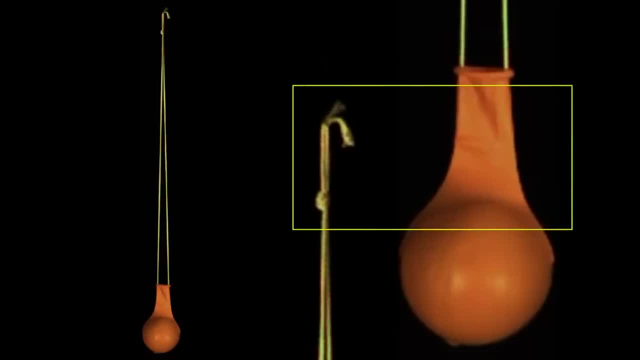 occurring only at the top of the string, which is almost immediately followed by motion at the bottom of the string. Because we have so few frames to work with, we can only estimate that the tension wave propagates at a speed somewhere between 1500 and 3000 meters per. 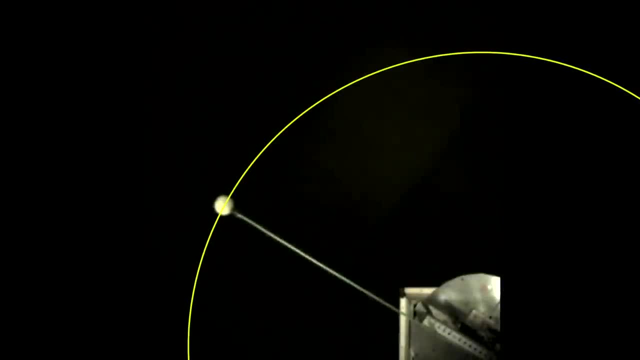 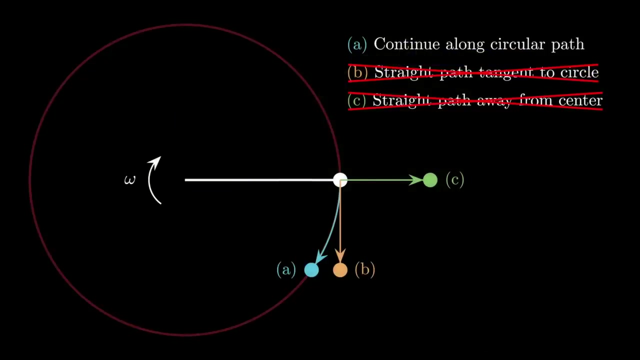 second. Unfortunately, this very large wave speed makes it impossible for us to capture the ball continuing to move in circular motion upon release, like we did for the slinky noodle and elastic cord. But hopefully I've already convinced you of the answer to our original question Immediately after releasing the string. a. 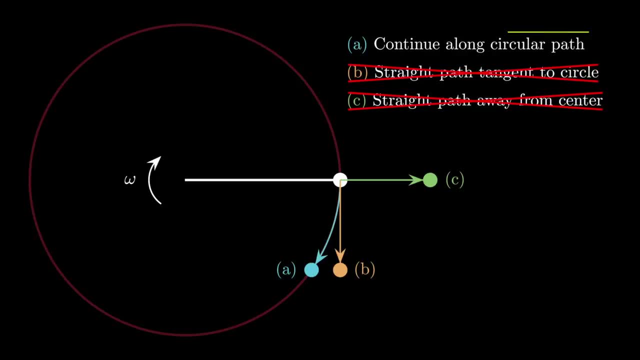 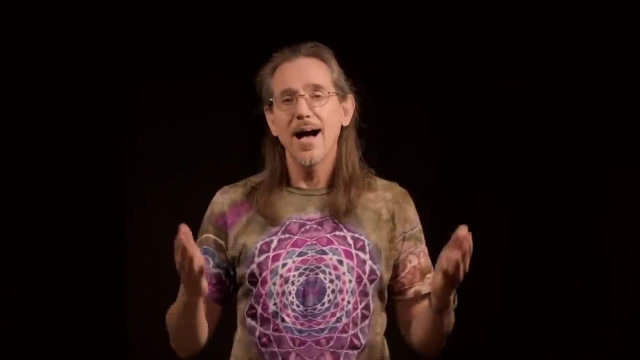 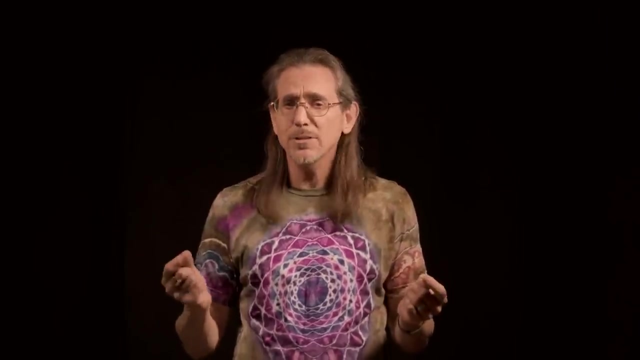 ball being swung around in circular motion will continue moving in circular motion, albeit only for a very brief time. I don't know about you, but I find this phenomenon to be quite fascinating. Of course, for a string length of one meter, the ball is only going to continue in circular motion. 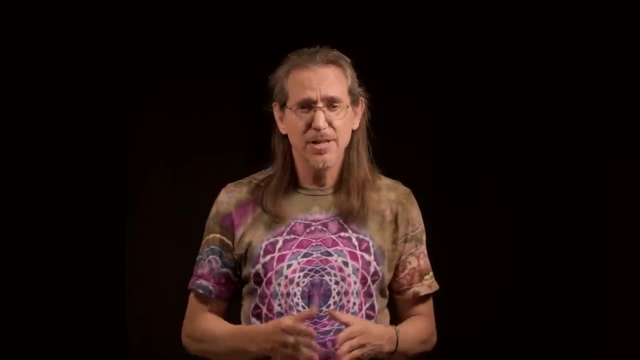 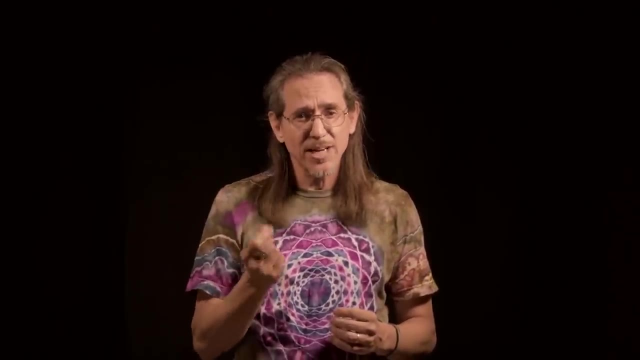 for about half a millisecond after being released. so you might think the effect on its trajectory is going to be relatively small. In fact, you might consider the trajectory to be well approximated by a straight line tangent to the release point And, to some extent, this: 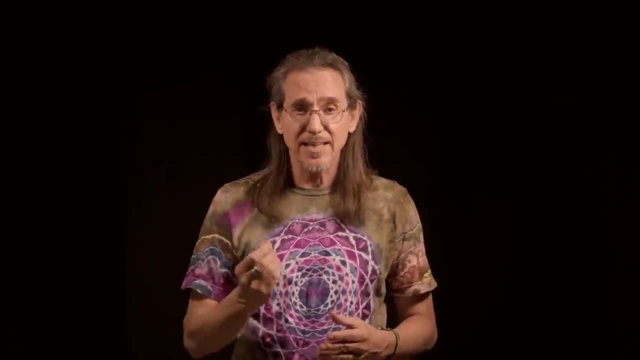 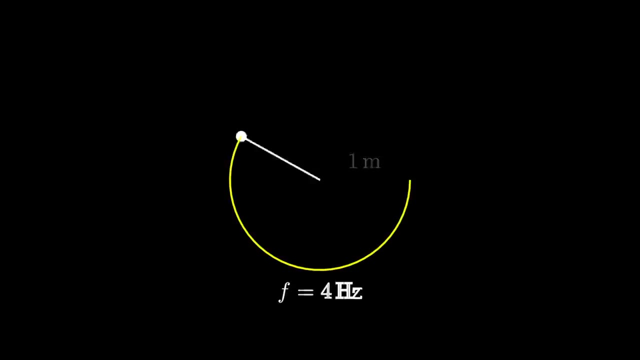 is true. However, the effect we've been discussing is larger than you might imagine. For example, if the ball is being swung around with a frequency of 4 hertz and is launched a total distance of 10 meters, the ball will actually end up more than 12 centimeters laterally from where. 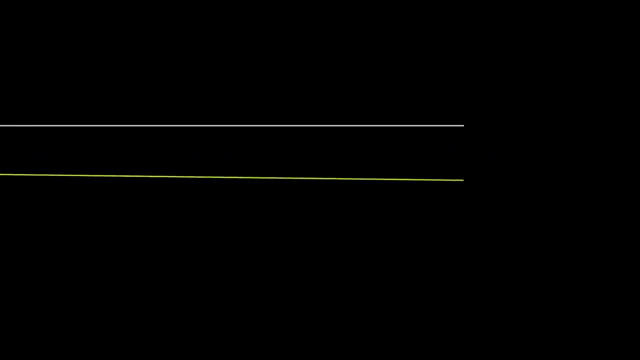 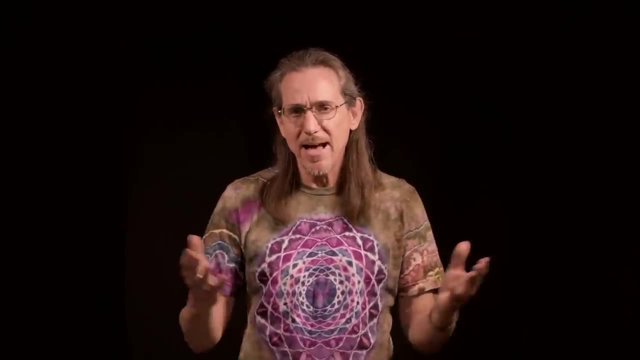 you would expect it to be if it was moving tangent to the release point. That's surprisingly significant. And finally, let me leave you with one last thought. Imagine that, somehow, the sun were to completely disappear from the sky. Imagine that the sun were to completely disappear. 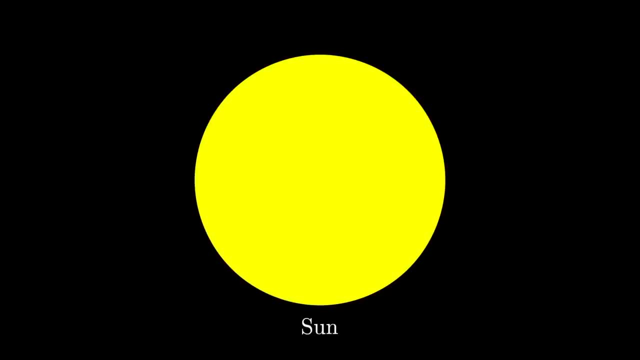 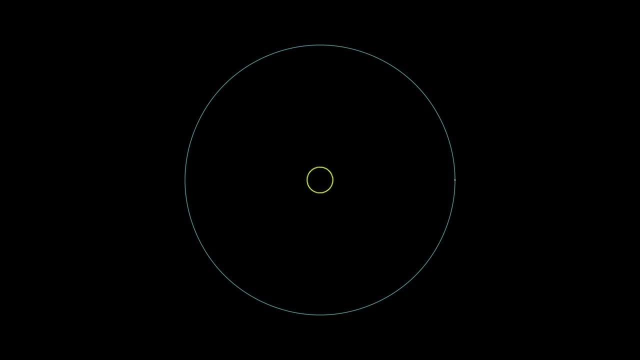 from existence. According to general relativity, gravitational changes travel at the speed of light, so the Earth would not feel the effects of that for about 8.3 minutes. Therefore, not only would we continue to see light from the sun for the next 8 minutes, but Earth.